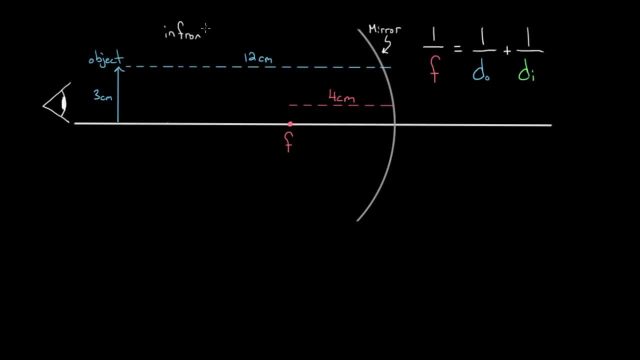 So this side over here is in front of the mirror- positive- And back here would be behind the mirror and that would be negative. So I've got some numbers in here already. Let's just solve this one. So what do we do? We're going to use this mirror equation. We're going to say that one over 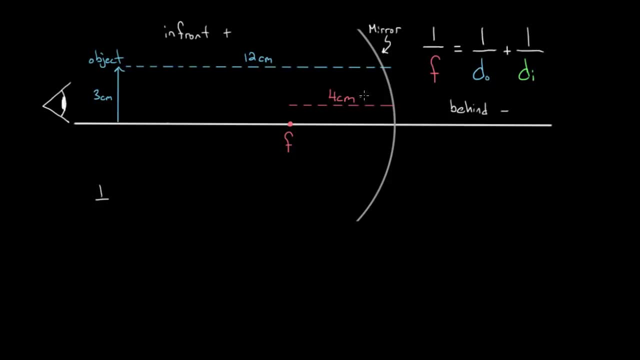 the focal length And already we have to decide on a positive or negative sign. So this mirror, the way it's shaped right here, based on how we're looking at it, is a concave mirror And, with the sign conventions we just discussed and the signs I'm using in this formula, concave mirrors. 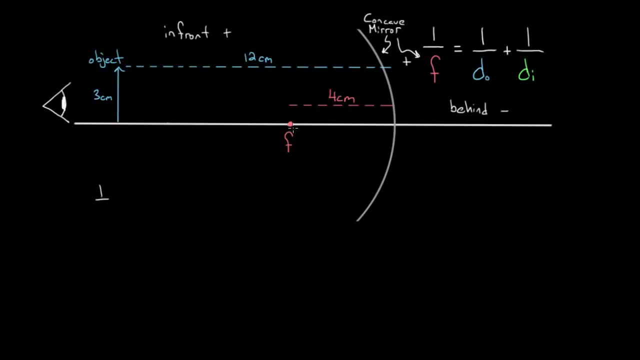 always have a positive focal length. So in other words, since this focal point is four centimeters from the center of the mirror, I'm going to have to plug in the focal length as positive four centimeters. Notice, I'm not converting. That's okay If you leave everything in centimeters. 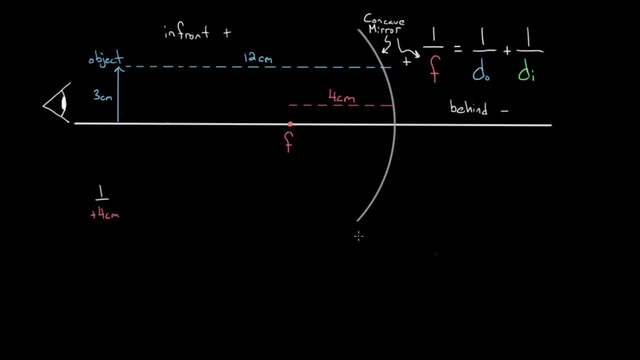 you'll just get an answer in centimeters. So it's okay, You don't have to convert as long as everything's in the same units, And we'll set that equal to one over the object distance. Just one other warning: Sometimes, instead of D? O, you'll see this as S? O for object distance, And that's. 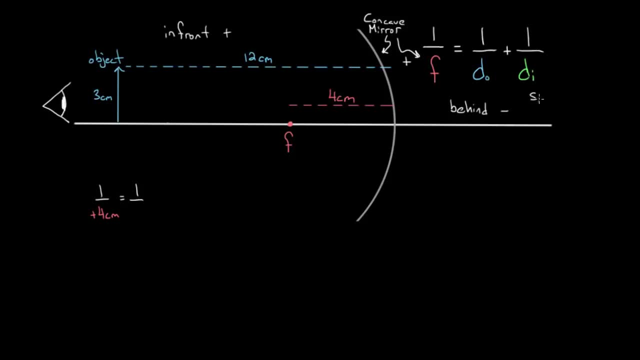 object distance, Or you might see D I as S I for image distance. It's the same thing, It's just a different letter. So the object distance again is on this side in front of the mirror, So it's going to be positive 12 centimeters, since it's located 12 centimeters from the center of the 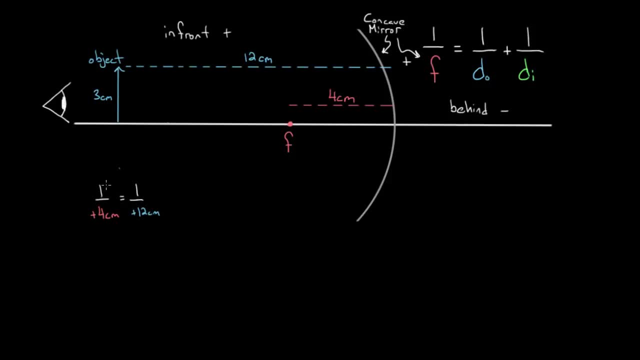 mirror. So there's also going to be positive 12 centimeters, And now we're going to add to that one over the image distance. The image distance we don't know. I haven't drawn the image on here. It's going to be a surprise. We don't know where this is going to be, but we can solve. 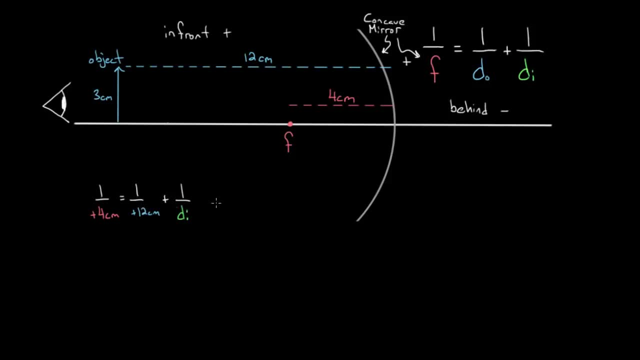 for it. So we can solve for image distance. I'll subtract one over 12 from both sides, which will give us one over four centimeters minus one over 12 centimeters, And that's going to have to equal one over the image distance. So one fourth you could rewrite as three twelfths, So three twelfths. 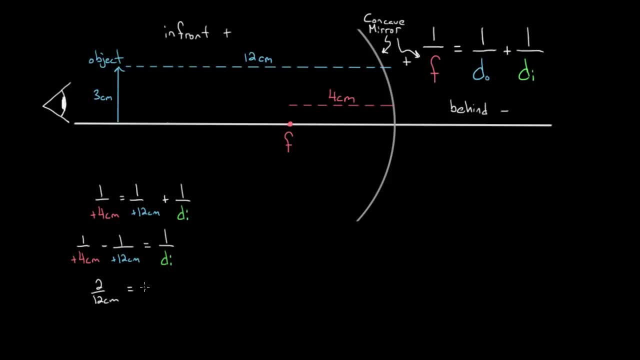 minus one twelfth is just going to be two twelfths, And that's going to equal one over the image distance. But two twelfths is just one sixth. So one over the image distance is just going be 1 sixth, but that's what one over the image distance is. 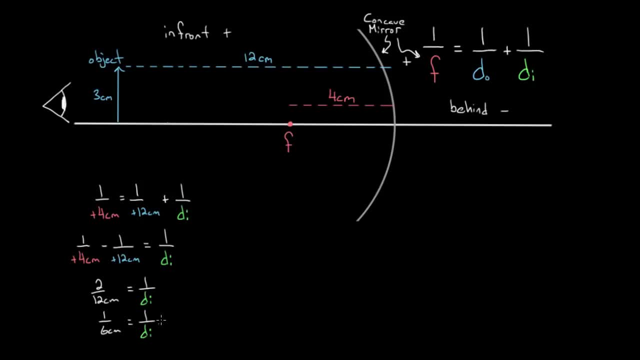 Sometimes people forget to flip this at the end. We don't want one over the image distance, we want the image distance. So finally you take one over each side and we solve and we get that the image distance is gonna be six centimeters. 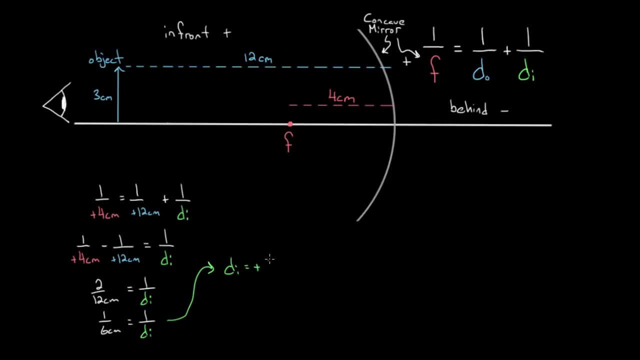 And it came out positive. that's important. This came out to be positive six centimeters, So where's our image gonna be? So, since this image distance came out to be positive, our image is gonna be in front of the mirror, So it's gonna be over here and it's gonna be. 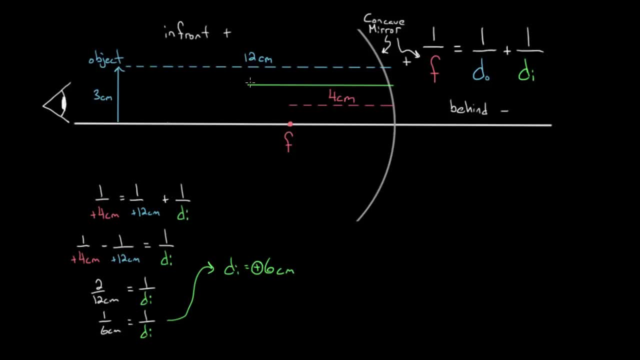 six centimeters from the mirror somewhere around here. So at this point, right here is where our image is gonna be, But we don't know how big it's gonna be, or whether it's right side up or upside down. To figure that out, we have to use a different equation. 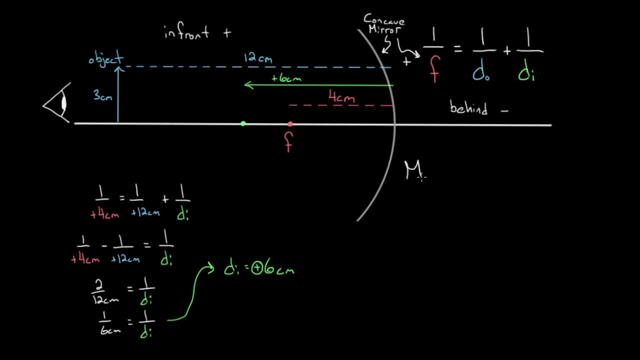 and that equation's called the magnification equation. It says that the magnification is equal to the height of the image divided by the height of the object, and that's equal to negative the image distance divided by the object distance. So it turns out: 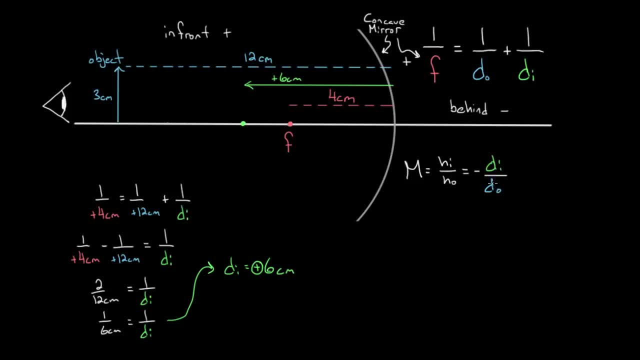 the ratio of negative image distance over object distance is always equal to the ratio of the height of the image over the height of the object. So what's the height of our image gonna be? Let's just solve for it. If we solve for the height of our image. 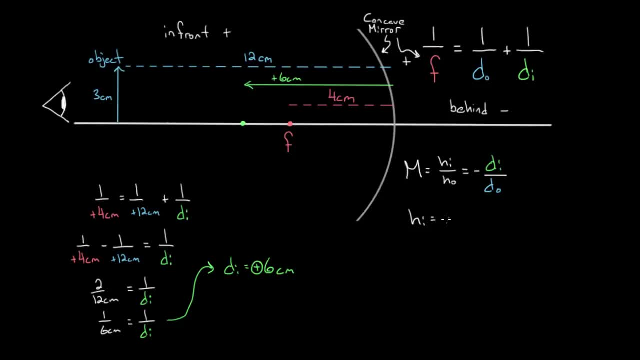 we get that the height of the image is gonna be multiply both sides by HO, we'll have the negative signs already here. so negative height of the object times this ratio of the image distance over the object distance. And now we can just plug in numbers. 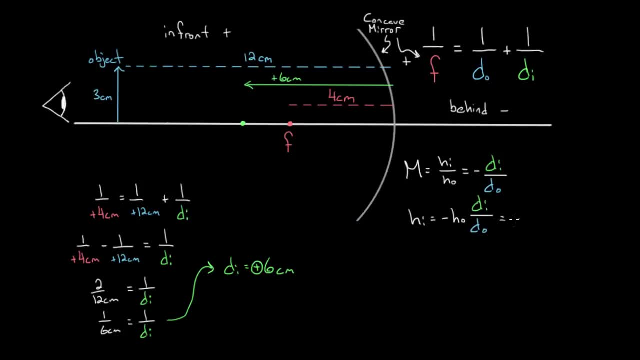 The height of the object. this is three centimeters tall right here. so it's three centimeters. so negative three centimeters times the ratio of the image distance was six. the object distance was 12. And so, if you solve this, 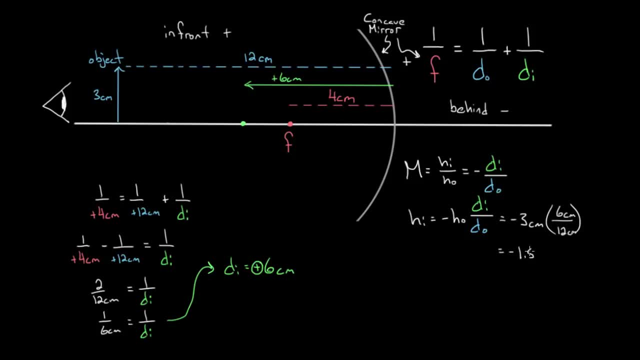 you'll get one half of negative three, which is negative 1.5 centimeters. The negative sign means that this image got inverted, So it got flipped over. It's gonna be upside down compared to what it was before And the 1.5 is how tall it's gonna be. 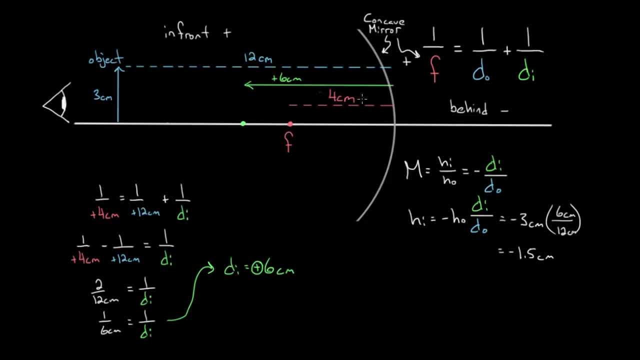 So what we end up with is an image six centimeters from the mirror and it's gonna be have a height half as tall, so 1.5 centimeters- and it's gonna be upside down because of this negative sign. 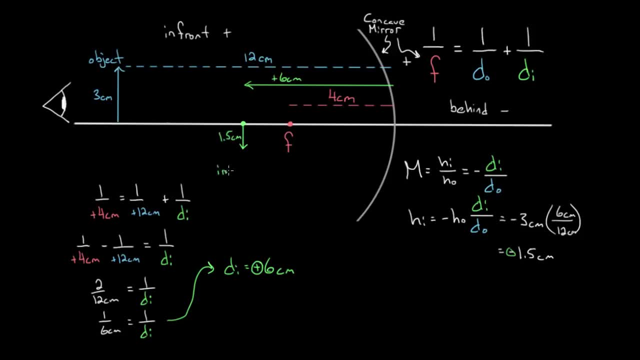 So it's gonna be 1.5 centimeters tall and upside down. That's what you're gonna see if you look into this mirror. It's like a fun house mirror. It's a weird curved mirror. You'd see an upside down image right here. 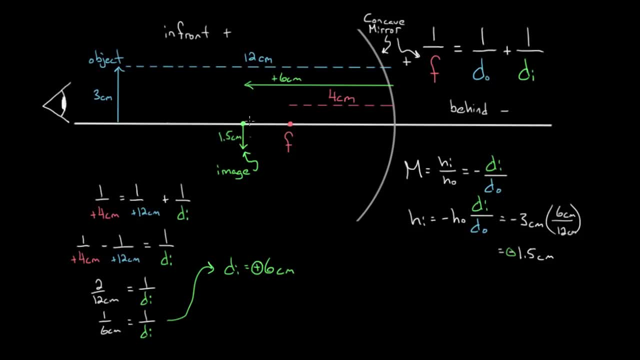 It might look like you could reach out and grab it, but it's gonna be an optical illusion. There's gonna be no object there, It's just gonna be the image of this object here. So that's an example Using a concave mirror. what would change? 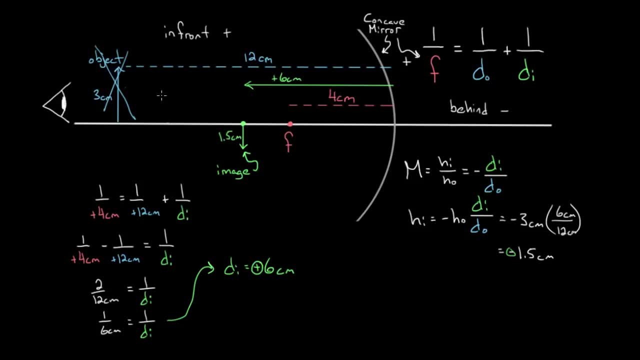 What if we did this? What if we took our object so say: we don't put it here anymore, We move it inside here. So instead of being at 12 centimeters, we moved it to like three centimeters. What would we do differently? 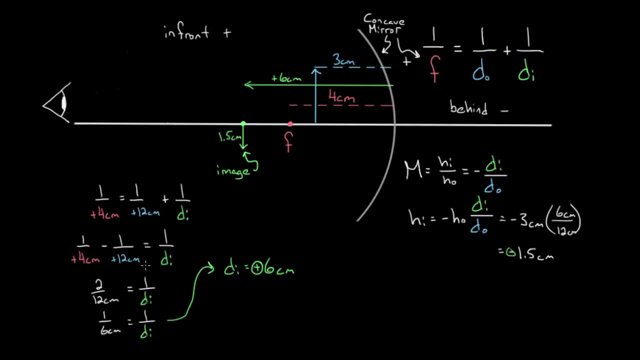 Everything would be the same. We just would plug in: instead of positive 12 down here, we'd plug in positive three. So the mirror equation works exactly the same. You still plug in. whatever that object distance is, You solve for your image distance. 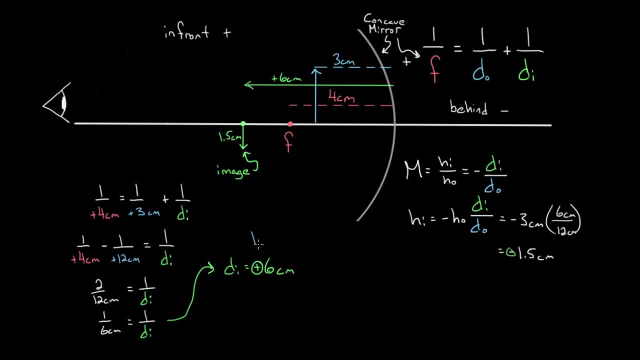 we're of course gonna get a different image distance, But whatever you get, that would tell you where the image is And then you would take that, plug it into the magnification equation if you wanted to decide how big the image is gonna be. 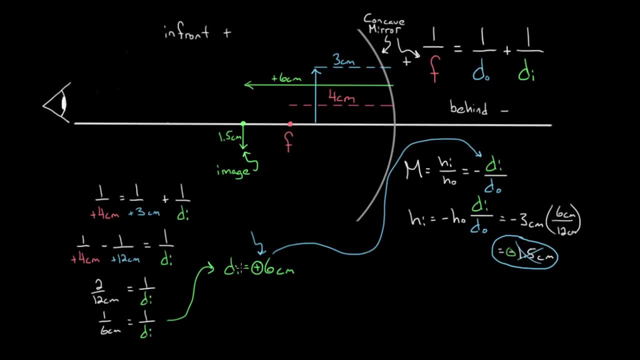 and whether it's gonna be right side up or upside down. So these numbers are gonna be different, but you would use this equation the exact same way. Now, what would happen if, instead of using a concave mirror, we used a convex mirror? 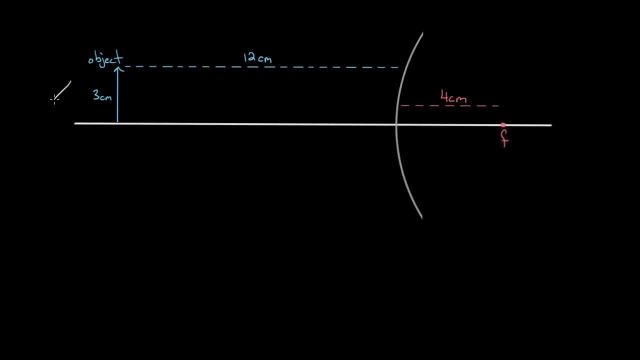 Let's say we used a mirror shaped like this. So imagine our eye again is over here, looking at this object inside of the mirror, and we're gonna see an image of the object. We're gonna see the object right here, but we're also gonna see the image of the object. 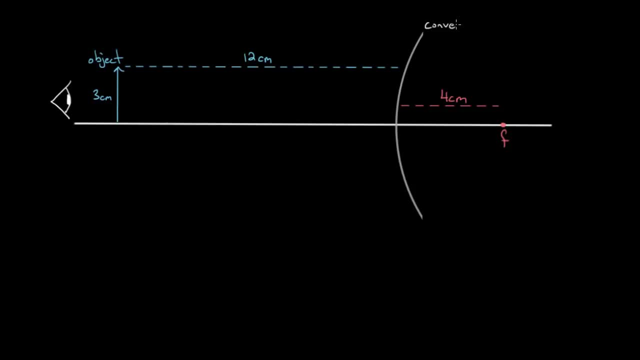 This mirror. this time, instead of concave, this is a convex mirror, So its focal length is behind the mirror. So what do we do now? to figure out where the image is? We again use the mirror equation. We're gonna use the same equation. 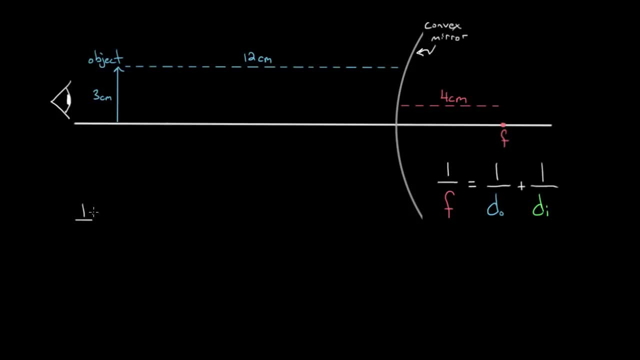 We're gonna have one over the focal length And again I immediately have to make a decision on the sign. With the convention that I'm using. this focal length is behind the mirror, So this focal length for a convex mirror is gonna be negative. 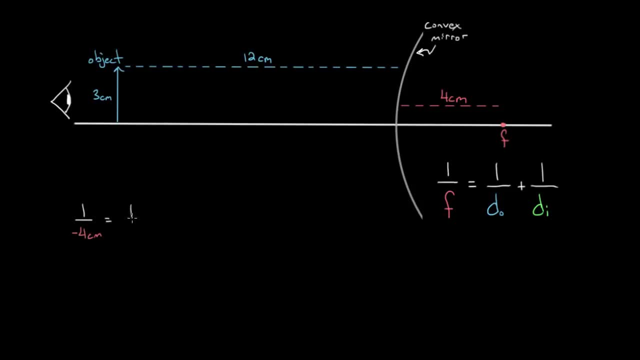 So this would be negative four centimeters And that's gonna equal one over the object distance. Well, again, the object is in front of the mirror 12 centimeters. so this object distance is gonna be positive 12 centimeters. And then we add to that the image distance. 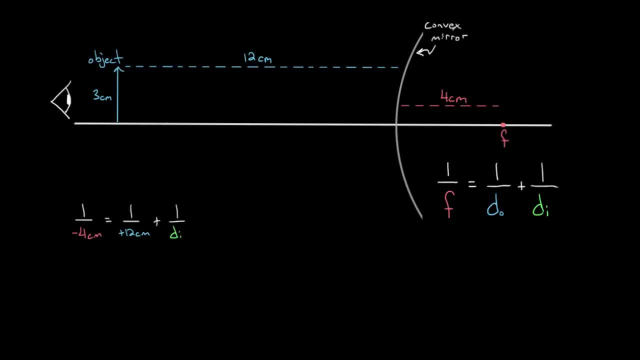 which we don't know. This is what we're gonna solve for. So this time, if we solve, we're gonna have one over negative four And again we have to subtract one over 12. And that's all gonna have to be equal to. 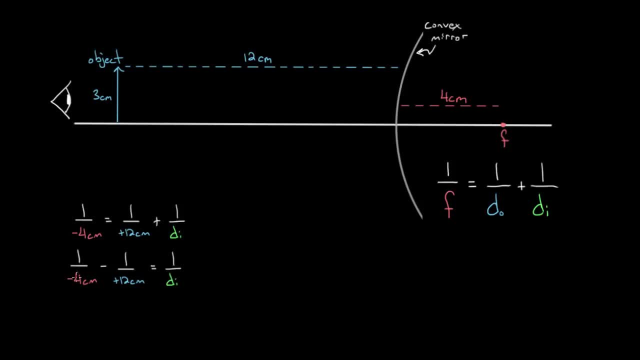 one over the image distance. So now on the left hand side we have negative 1- 4th, but that's the same as negative 3 12ths. So negative 3 12ths minus 1 12th is the same as negative 4 12ths. 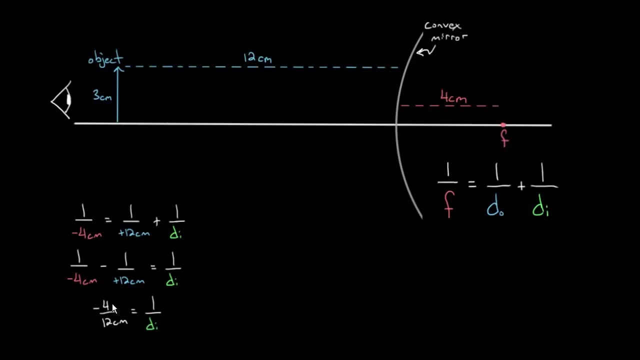 And that's gotta equal one over the image distance. But negative 4- 12ths is the same as negative 1- 3rd. So one over the image distance has to be equal to negative 1- 3rd. And if we flip that over, 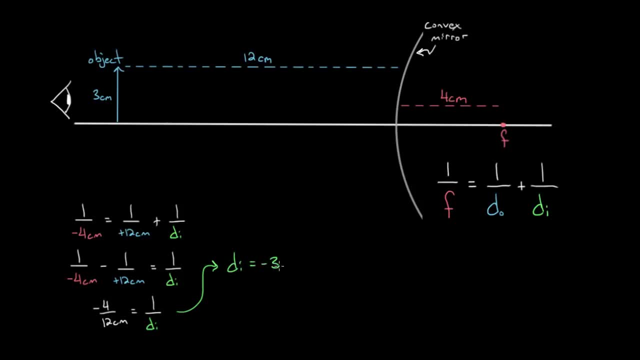 we get that the image distance, finally, is gonna be negative three centimeters. So in other words, this here is negative 1- 3rd. So when you flip that over, you get that the image distance is negative three centimeters. Where's this image gonna be? 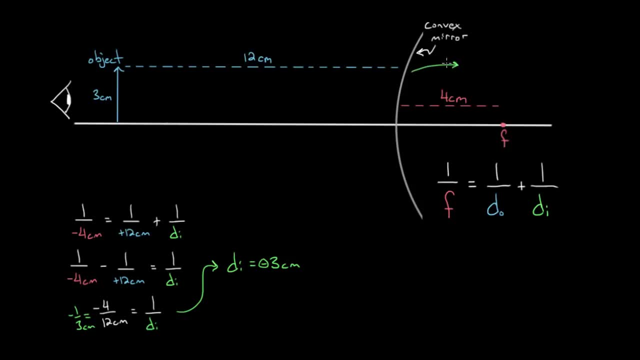 Well, since it came out negative, that means it's behind the mirror, Cause that's the sign convention we're using, So it's gonna be three centimeters behind the mirror, So it's gonna be like over here about at this point. 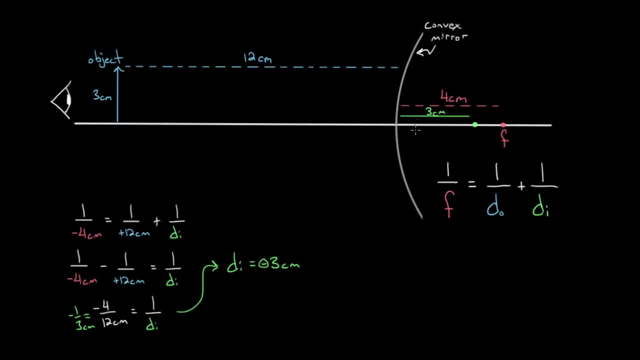 right around here, somewhere Three centimeters behind this mirror. And again, if we wanna figure out how tall it's gonna be, whether it's right side up or upside down, we're gonna have to use the magnification equation, And that magnification equation looked like this: 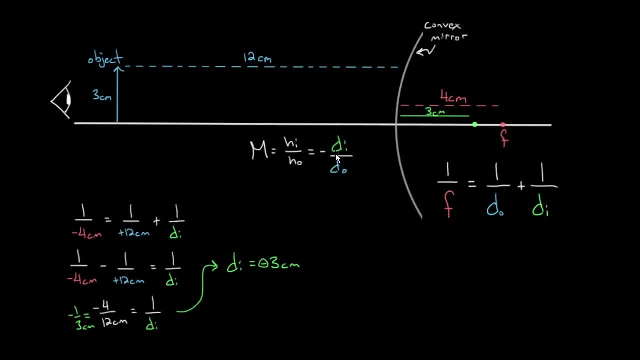 It said that the height of the image over the height of the object had to be negative: image distance over object distance. So let's just see what this right hand side's gonna be If we just set this equal to. it's gonna be negative of negative three. 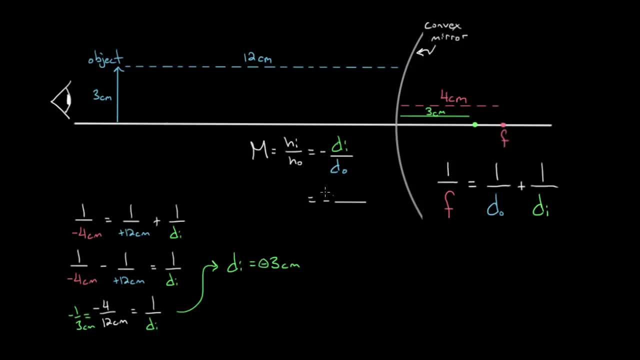 is the image distance. So I have to plug in the negative three And you keep that negative in there. This negative out here comes along always. but now we have another negative inside of this image distance of negative three And the object distance again. 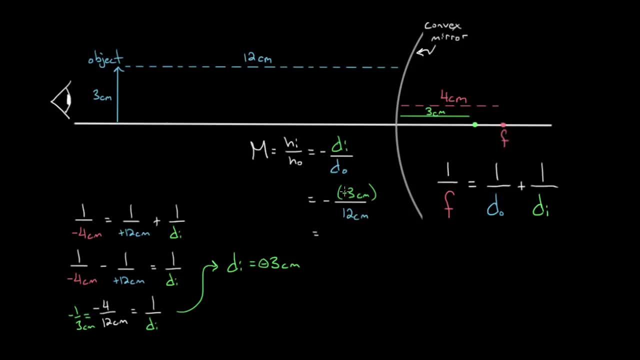 was 12 centimeters. So what are we left with? We get negative of negative, three, which is positive, three over 12, which is positive, 1, 4th, And the centimeters cancel. So what this ratio tells you. 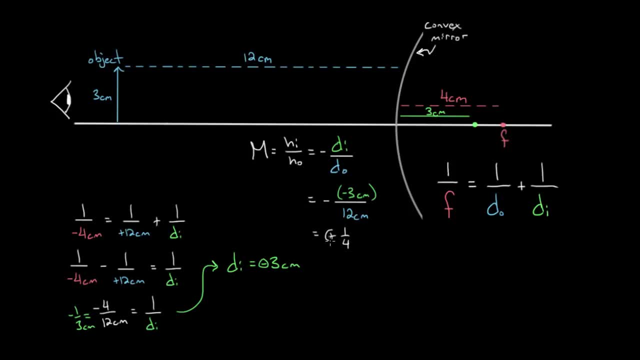 which is the magnification is that the image is not gonna be inverted. This positive means it's gonna be right side up And the 1 4th ratio means it's gonna be 1 4th as large The image. I should say: 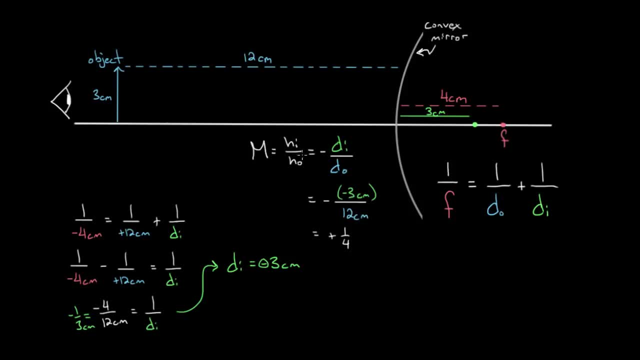 is gonna be 1, 4th as large as the object is gonna be, And the reason is this ratio is equal to height of the image over the height of the object. So, in other words, if I can multiply, if I wanna multiply, both sides. 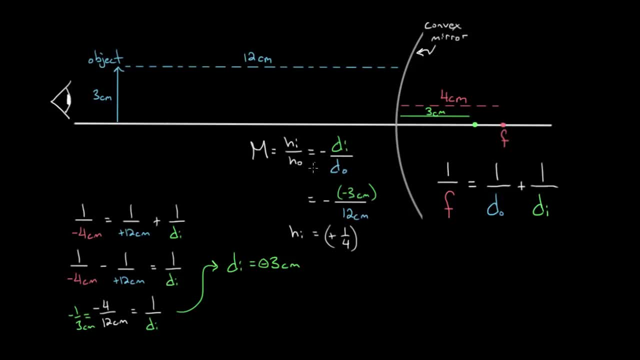 I can say that height of the image is equal to positive 1, 4th times the height of the object. Well, the height of our object was three centimeters in this case, But whatever your height of the object is, you multiply it by this ratio of negative d over d o. 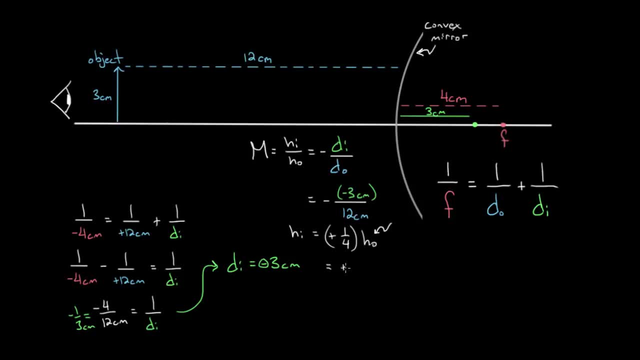 and you get what the height of the image is gonna be. So we're gonna get 1 4th of three. So we get positive 3 4ths of a centimeter. So it's gonna be tiny. This is gonna be little. 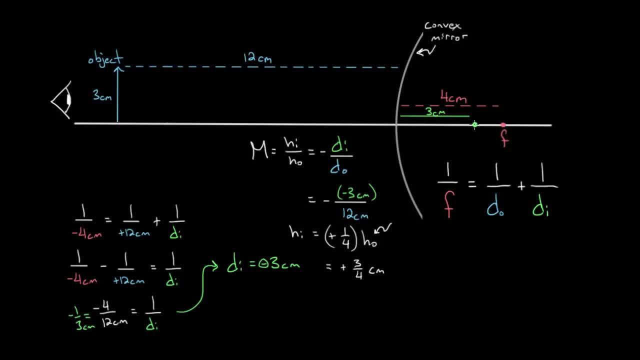 Little image. It's gonna be right side up, So it's gonna be right here, but it's gonna be teeny. It's only gonna be like this: 3 4ths of a centimeter tall. That's what our image is gonna look like. 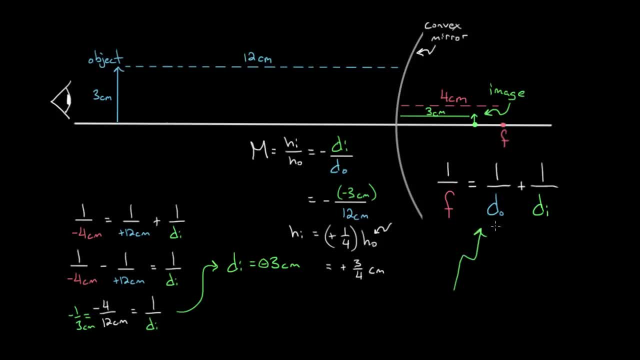 So, recapping, you can use the mirror equation to figure out where the images are gonna be located. The sign convention we're using is that objects, images and focal lengths in front of the mirror are gonna be positive. Anything behind the mirror is gonna be negative. 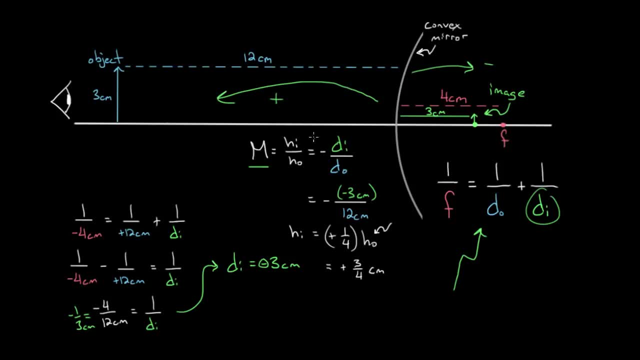 And you could use the magnification equation to figure out how tall the image is gonna be relative to the object by taking negative the image distance over the object distance. 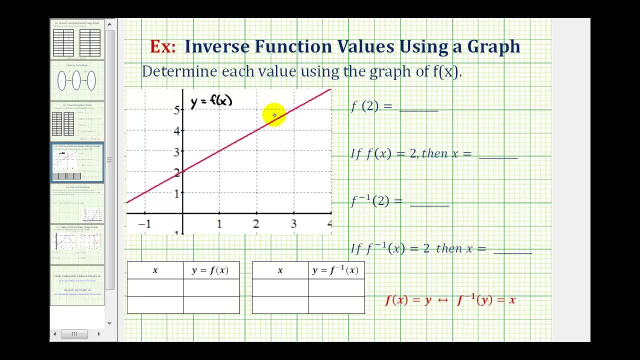 Here we're asked to use the graph of function f of x, graphed here in red, to determine the values here. on the right Notice, two of these involve the function f and two involve the inverse of function f. To evaluate f of two, we need to recognize that this two is the input or the x value for function f.